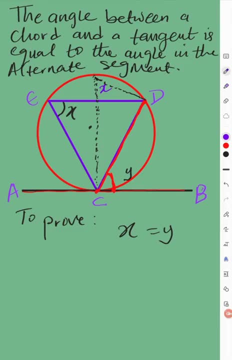 There is a theorem which says that there are equal which is angle in the same segment. Okay, So that particular angle is now an X. Remember also that there is another theorem that says that the angle between a chord and a radius is a right angle. 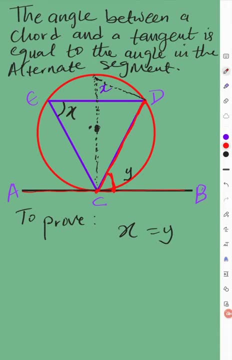 So from here the center down to this circumference is X, So this is a radius, And because it is a radius, this angle here is 90 degrees. If this is 90 degrees, it means that here also, that this is also 90 degrees. 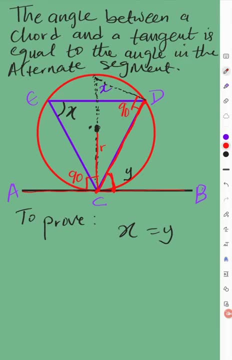 The reason why here is 90 degrees is because we call it angle in a semicircle. The angle in a semicircle is equal to 90 degrees. Since we have drawn a diameter that will be 90. That means this small angle here will be 90 minus Y. 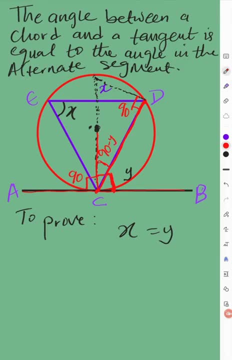 Why will it be 90 minus Y? Here is also 90, a radius and a tangent makes angle 90 degrees, So here is 90 degrees. Alright, So sorry, here is 90 minus X and not 90 minus Y. 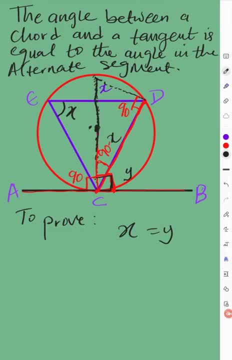 The reason is because we have this triangle here which I'm shading. This is a triangle, And the sum of angles in a triangle is 180 degrees. Already, this angle is 90.. When you remove the 90 from 180, you are left with 90. 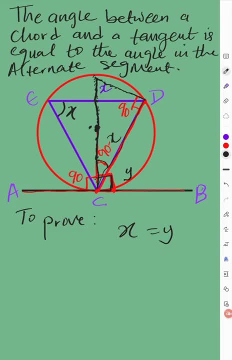 90 degrees. Hence the third angle will be equal to 90 minus X, since here is already X. So since this is 90 degrees, the angle here is a right angle. So you can now add. look at the angles I'm talking about. 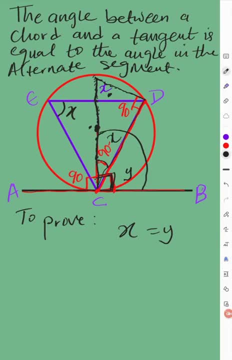 These angles- here they are right angles. angle between a radius and a tangent. So I can now comfortably write that 90 minus X plus the Y is equal to 90 degrees. Alright, Call it. angle between a chord and a tangent. 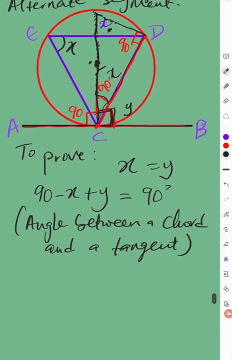 The angle between a chord and a tangent is 90 degrees. Therefore we can now, because we are looking for the value of Y, let's make Y the subject Y becomes 90 degrees. is here. This 90 crossing over becomes minus 90 and the negative X crossing over becomes positive X.